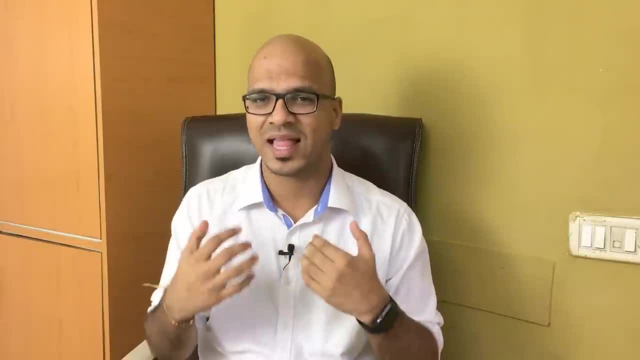 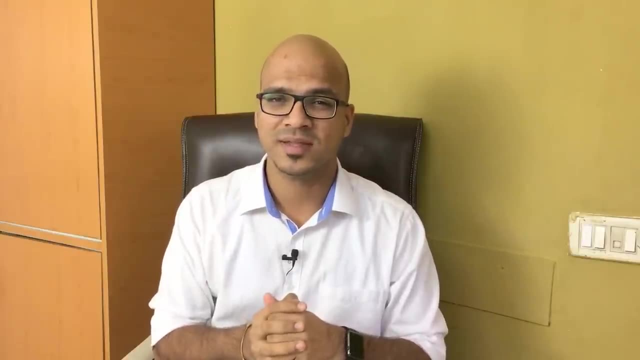 day they are adding new features. so if you want an application as a client, if you're going to a vendor and say, hey, I want a software, if a vendor says we will give you the entire software in one year, that's a very big time. what you want is: 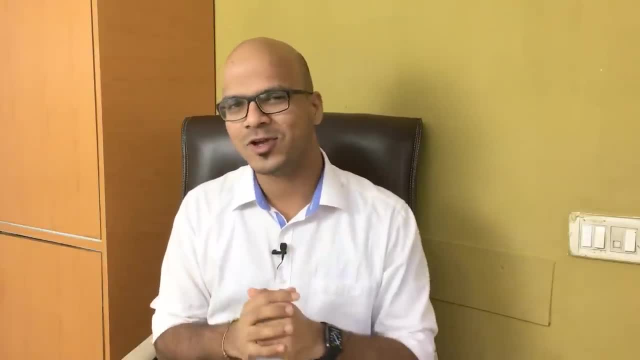 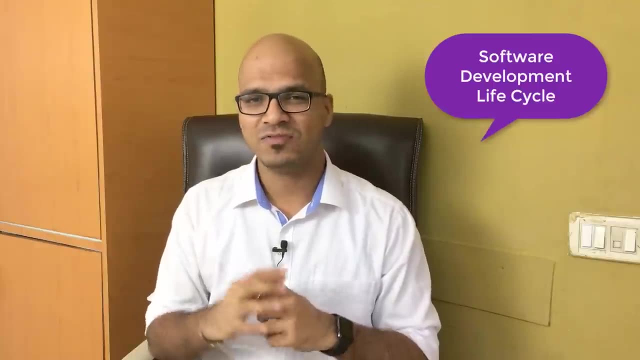 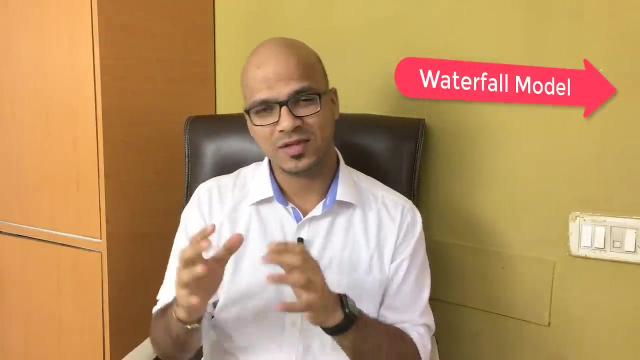 you want your software instantly now. if you go back to your college days, you know we have a concept of software development lifecycle in your software engineering and one of the methodology which we use is called as waterfall model, which is, you know, in waterfall what we do, we have whenever. 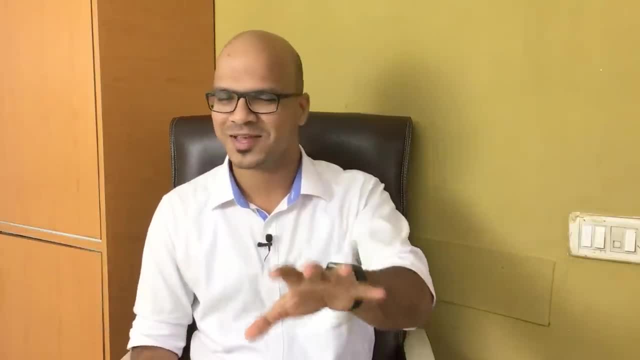 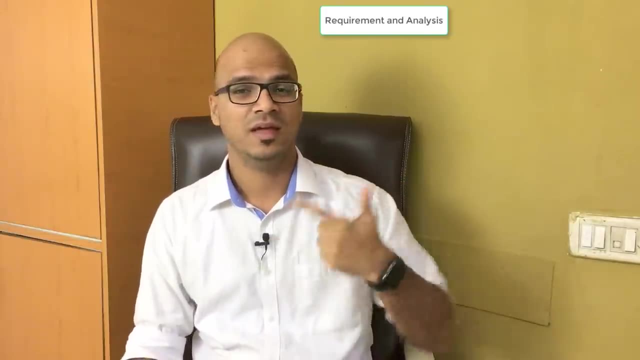 we want to make a software. we follow some steps. now your favorite those steps right, I know how how much you love those steps. the first step would be requirement gathering. then you have to analyze. that did analyze everythin. you have to design the software. you have to code this software. you have to test. 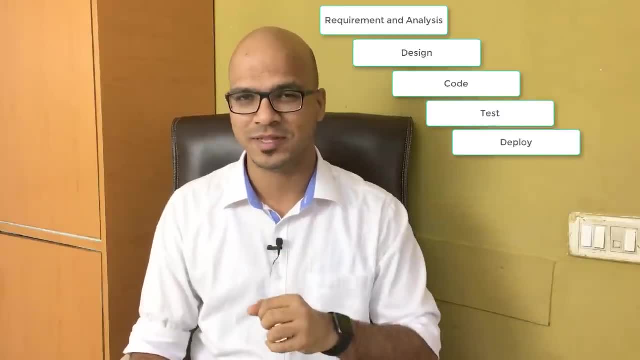 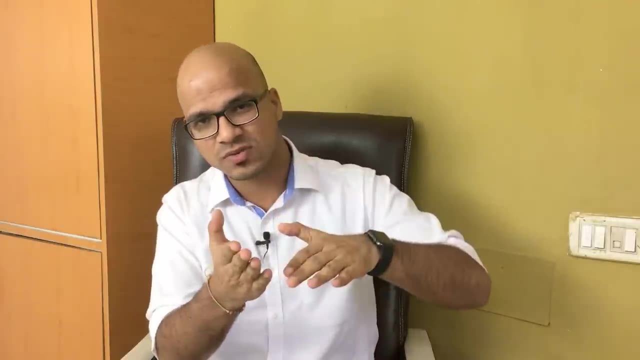 the software you have to maintain it. oh, you have to deploy first and then you will maintain it. right, so that those are the steps. now what happens, you know, in waterfall. So after you switch your phase, let's say from requirement phase, if you go to analysis and let's say if you go to design, now you cannot go back. 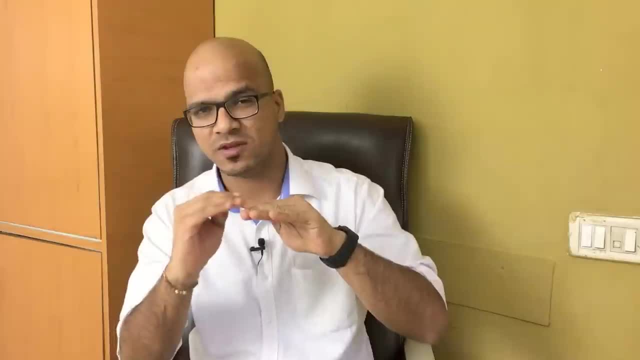 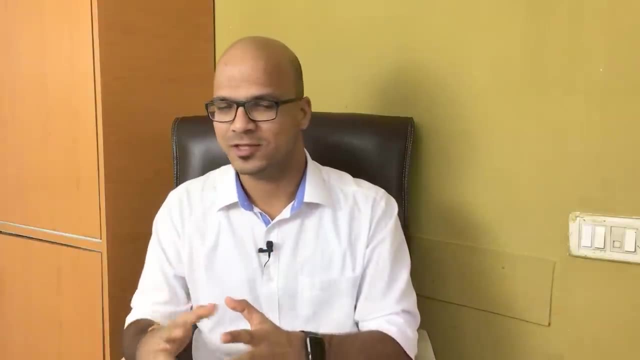 Let's say, if you go to testing field or testing phase the moment you get into testing phase, you cannot go back. So let's say, in six months you have done with the coding and now you're testing it. So your client comes to you and say, hey, developer or hey team. I want to make some change. 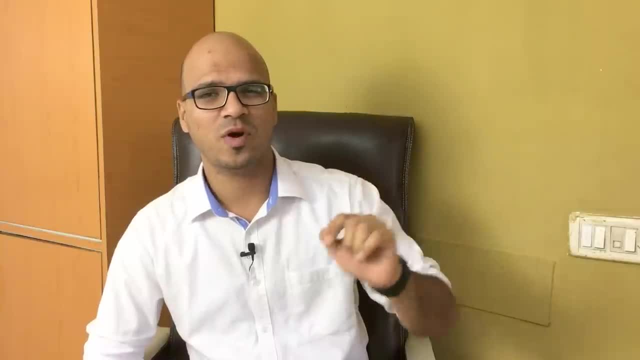 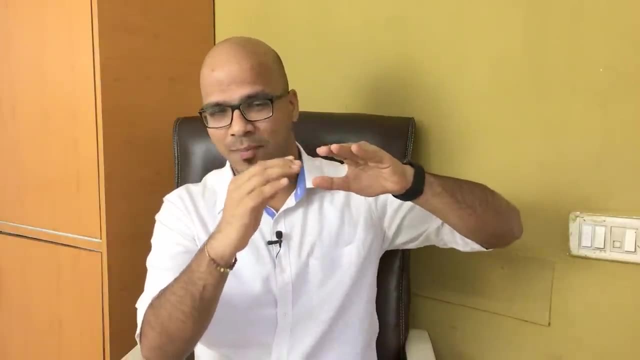 You know, Paytm or WhatsApp has added new features. I want the same feature now. Now can you do it In waterfall. what happens is the moment you get the requirement. you have to. first of all, you have to get the entire requirements right. 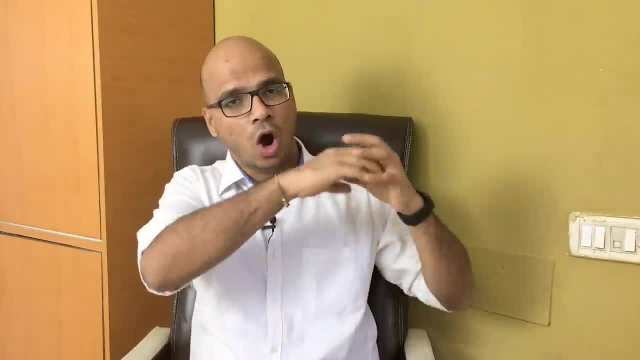 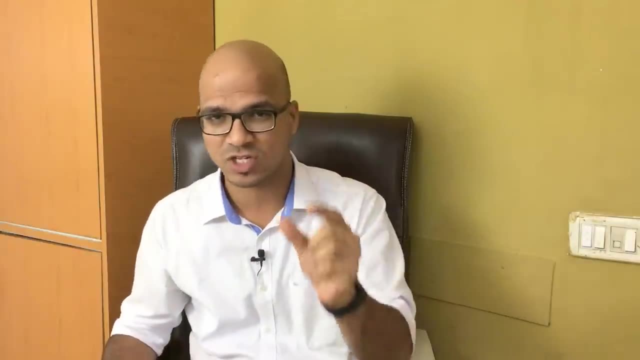 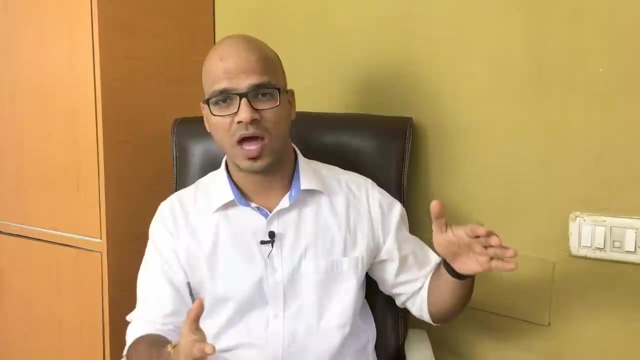 You cannot say: I will get some requirement later, So you have to get all the requirements and then only you can start Now. in the initial requirements it was not there, right, So that particular change was not there. So what you will do now? you will say, hey, client, I cannot change the code now because we got the requirements. 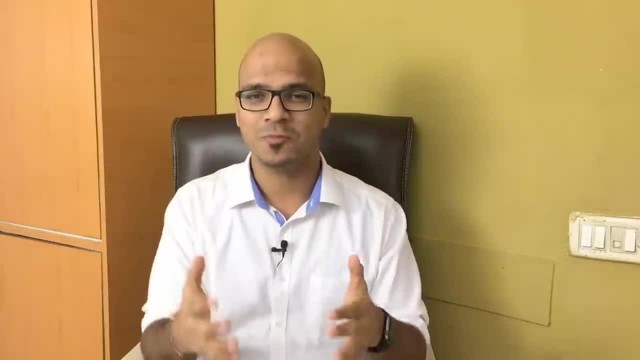 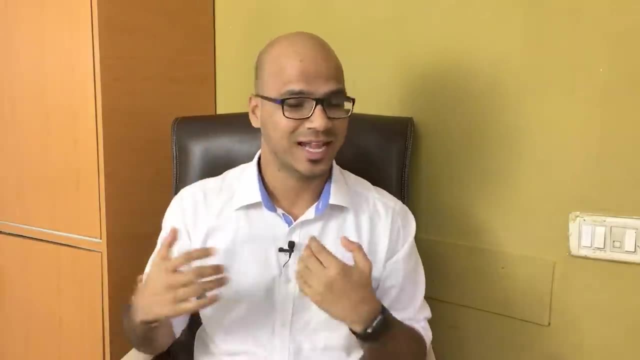 We have done with the coding phase. Now we are testing it. Now it's not possible. It's not possible for us to change anything in the software because, trust me, when you build a software, you build a software like House of Cards. 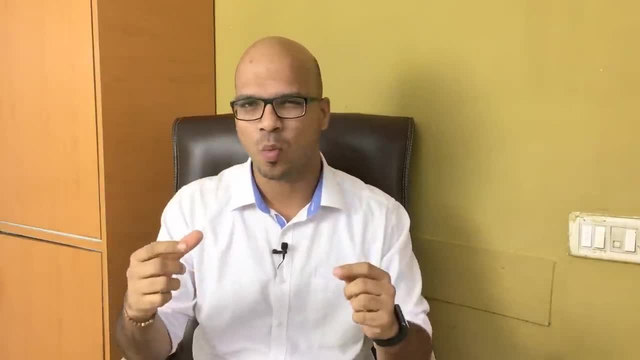 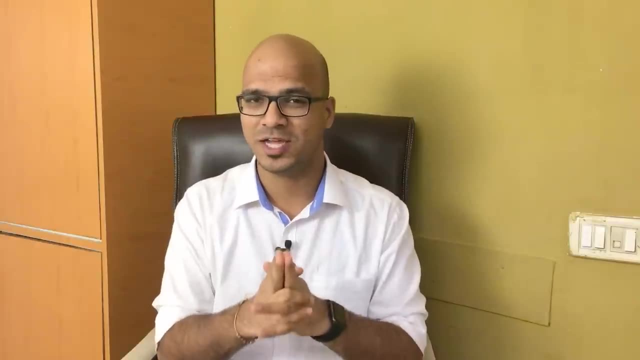 That's how I used to build software House of Cards. If you make one change somewhere, everything will fall, and that's the issue. So when you build a software, you have to make sure that it should be possible for you to make changes. 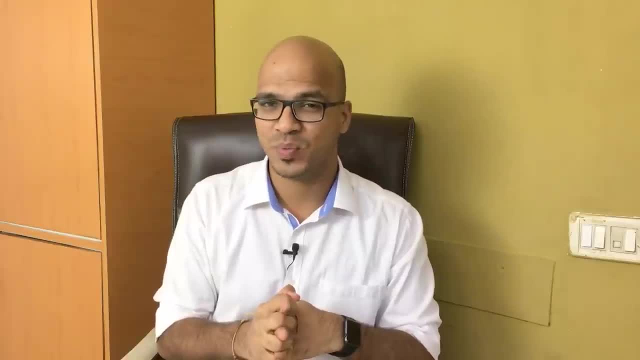 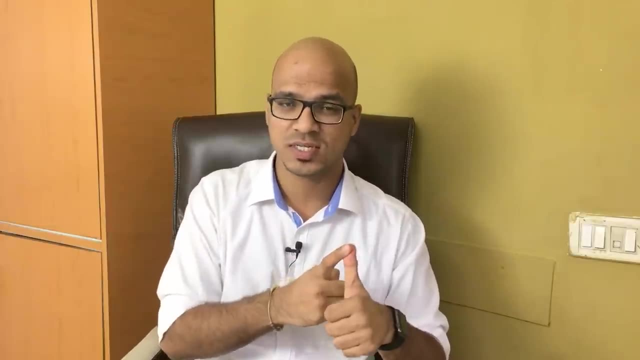 But unfortunately, if you follow waterfall you cannot change something in between. So there are some issues with waterfall. By no means I'm saying waterfall is bad, But then waterfall has some issues. The first issue is the time. to market is very slow or low, right. So if you want to build a software now, it will take some time to build the entire software and the market is somewhere else in that one year or two years. So if you want to build your own app now, start with the smallest part. 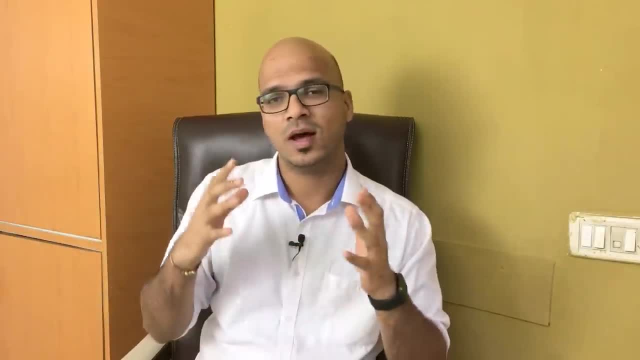 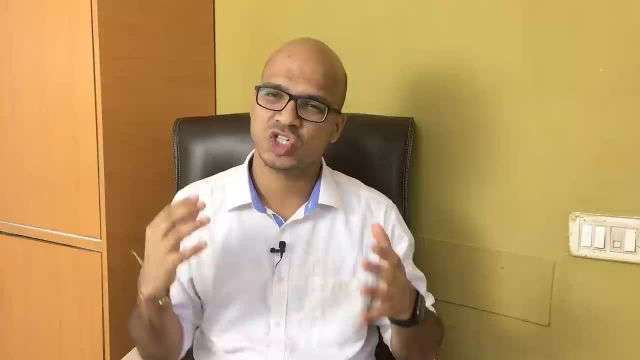 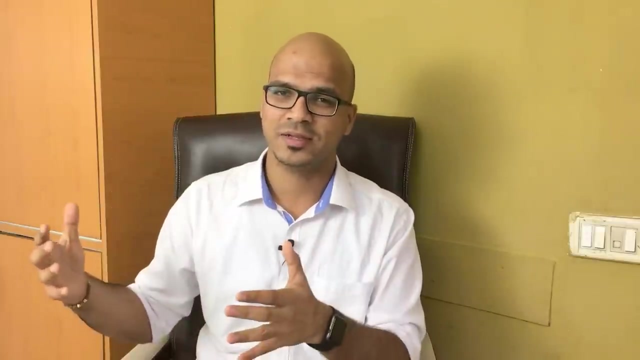 Don't wait for the complete application. Second thing: in waterfall, if you want to make changes, it will be very difficult. See, you have to understand your client and you have to understand the market. Market is changing very fast And, of course, if the client is investing his money in the software, of course you want to provide the client what it needs, right? 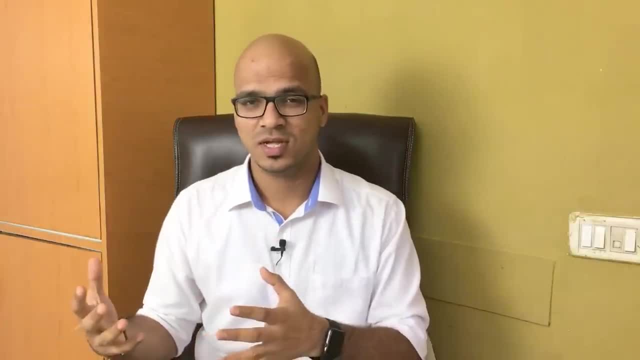 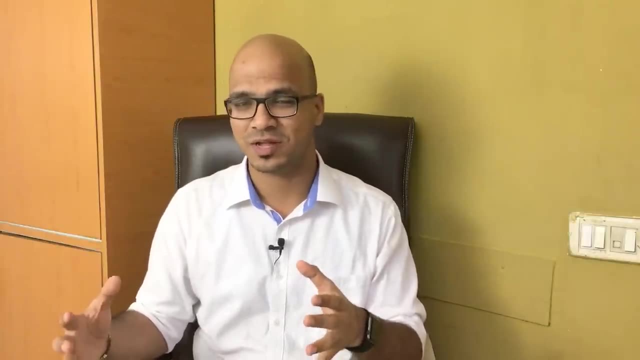 So you have to make sure that you accept the client changes. So this problem is there from a long time, you know. in fact, software industry is very new. OK, when you say new, it's there from last 30, 40 years now. and talk about other industries like banking industry, factories, constructions. 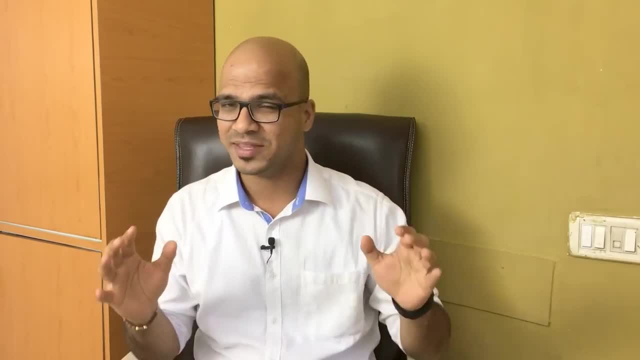 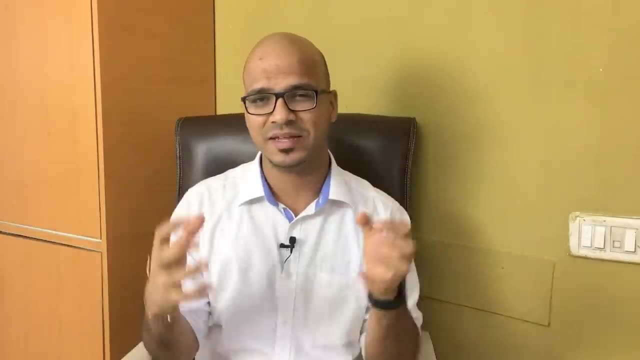 They are there from 100 years right, So they are very old. IT is very new. So the group of people- 17 people, they they came together and they created, so they were discussing about this. How can we solve this given problem? 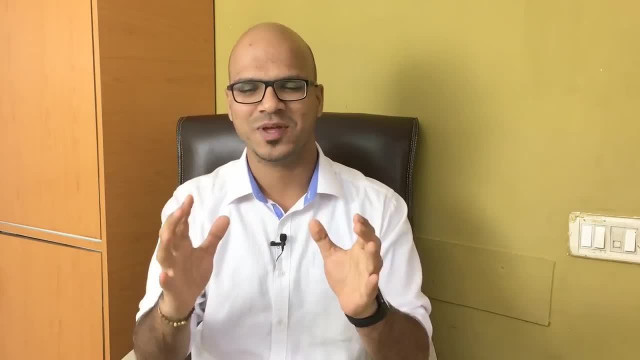 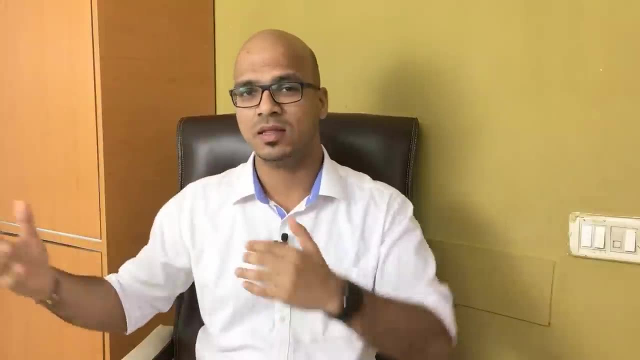 So they came together and they started giving some philosophy. And, trust me, that's what elder people do, right? So as a new generation, we don't do stuff as they want. So they have seen the entire world right, So they give their philosophy. 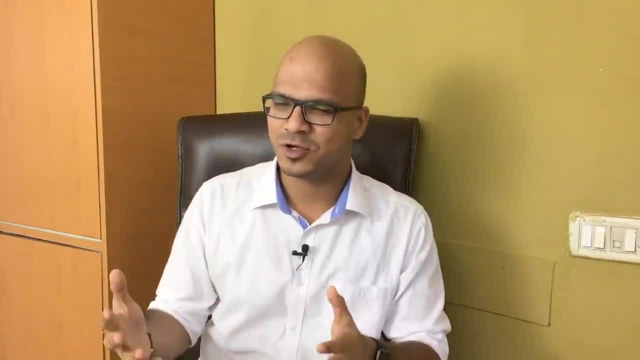 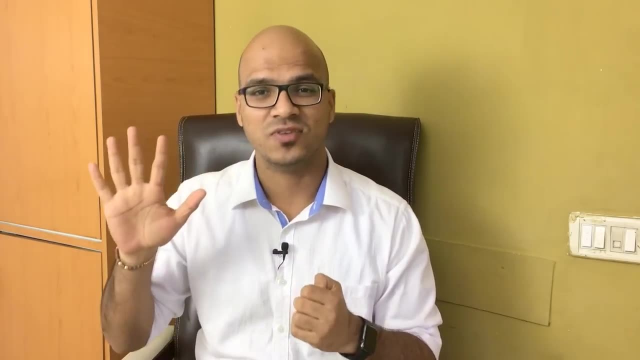 This is what you should do. This is what you should do, And not exactly you should do, but this is what you can do to achieve something. So, these 17 people, they have given some what you say philosophy, and they named that philosophy as Agile. 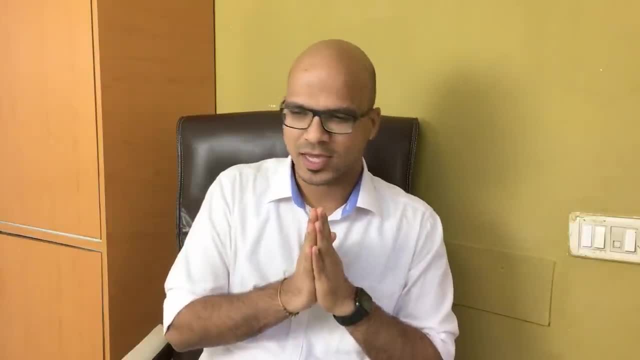 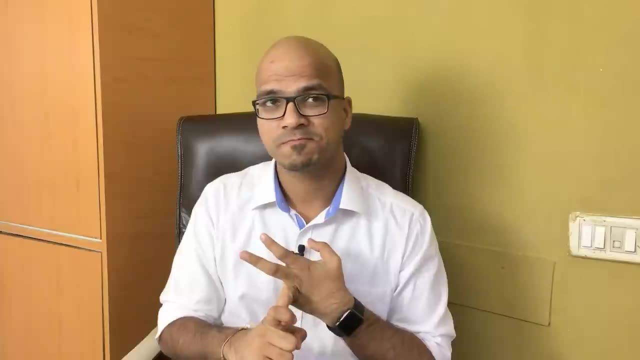 Now the question arises what they did. OK, so let's say, if they want to give a philosophy, what is the best way to give it? You can write a book, You can make a video, But the problem is, if you write a book, it will be a very big book, right? 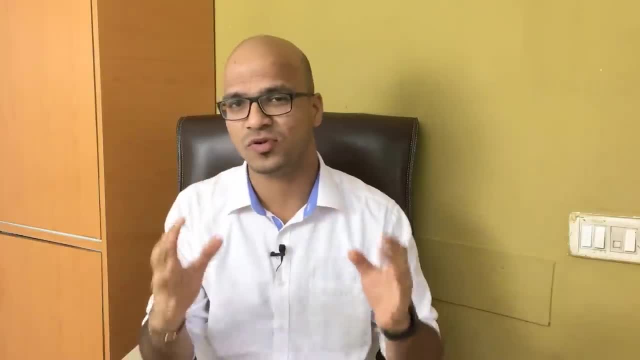 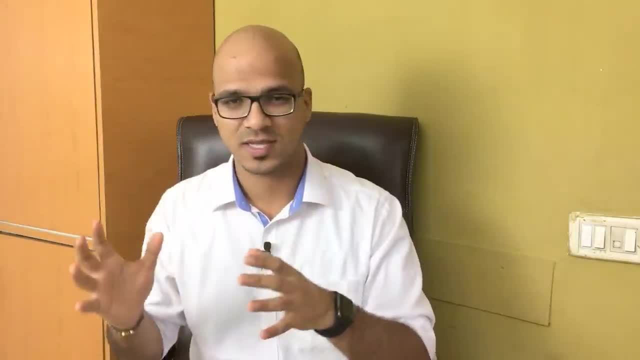 And if you ask a new team- hey, from now on, instead of using Waterfall, you should use Agile- They will say no, because changing your process is very difficult. So what I did? they said: OK, we will give you some manifesto. 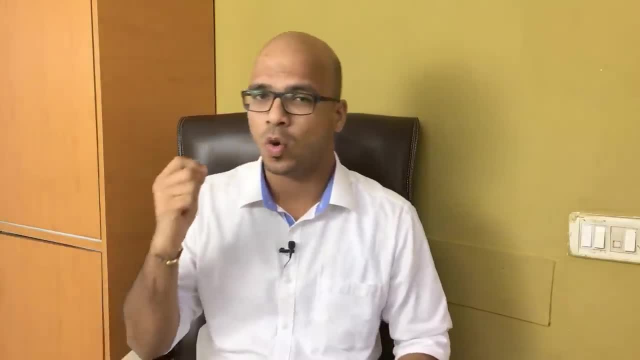 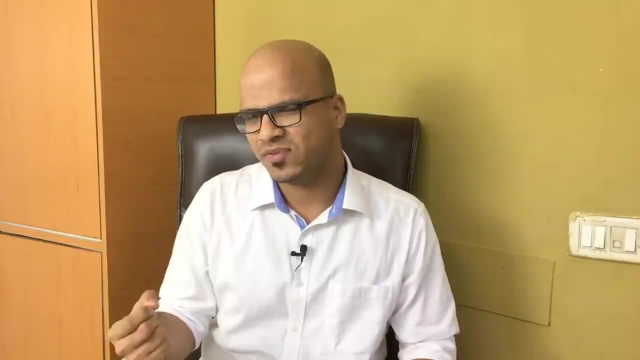 So we will give you a manifesto. Based on that manifesto, what you can do is you can just modify it or you can use it as per your way. So they've given the manifesto and now it's dependent upon you how do we implement it. 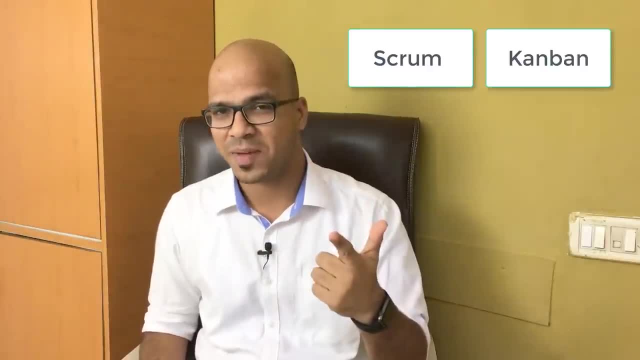 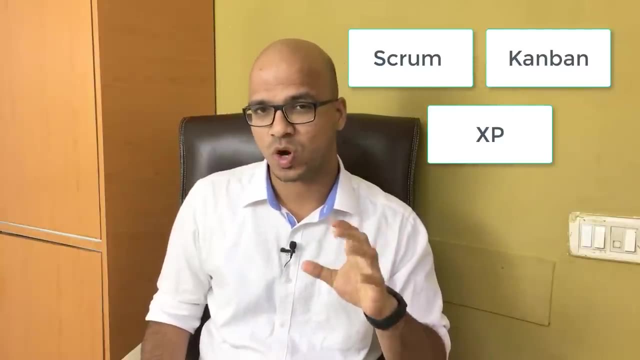 So there are multiple implementations for this. We have Scrum, We have Kanban, We have Extreme Booking, We have Extreme Booking, We have Extreme Programming. So there are lots of implementations for Agile. So now the question arises what they have given. 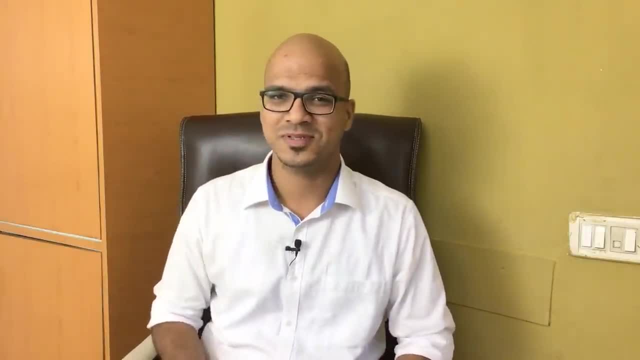 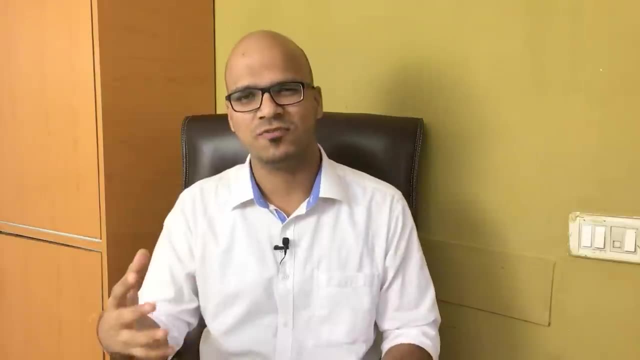 So they have given two things: the values and the principles. So if you can use those, or if you can implement those values and principles, you are doing Agile. Oh, there's a difference between doing Agile and being Agile. So, especially new teams, they start doing Agile. 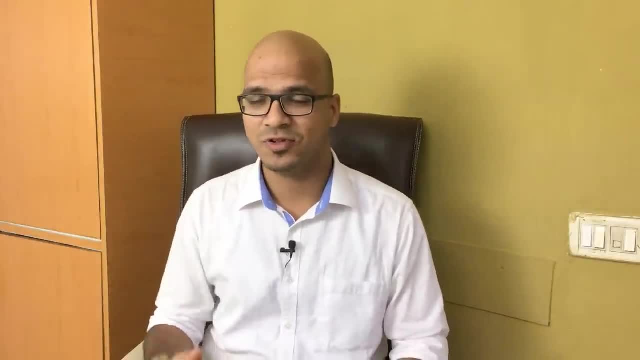 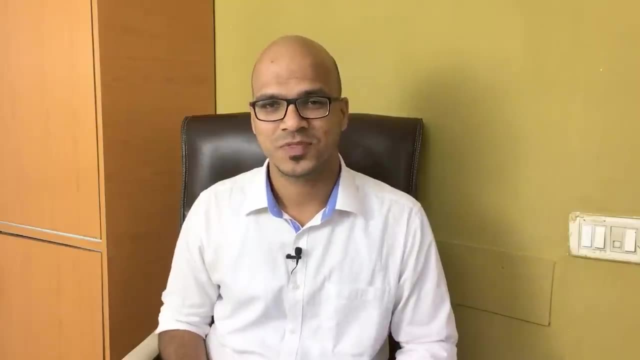 But it takes some time to actually be Agile, And if you really want to make good software, you have to be Agile. Now the question arises: what is those four things, Four values and twelve principles. So let's start with the values. 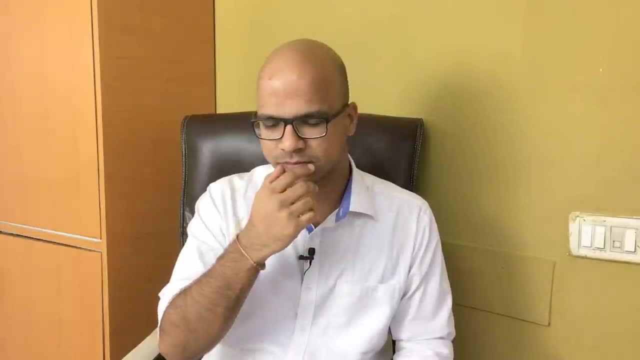 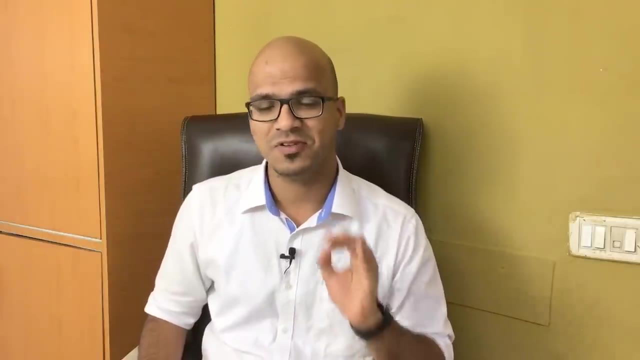 Now, before starting with the values let's talk about, again, go back to waterfall. In waterfall, what happens is we focus on some stuff. Example: in waterfall we focus on process, We focus on tools, We focus on documentation. 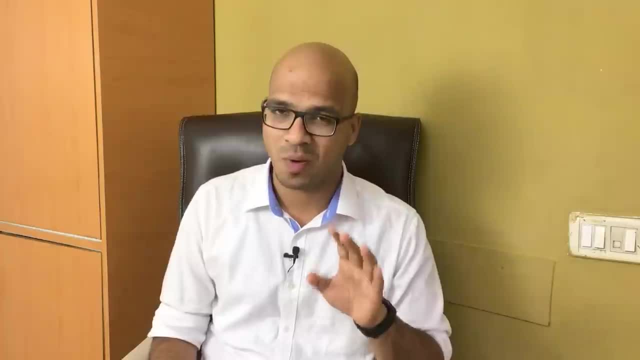 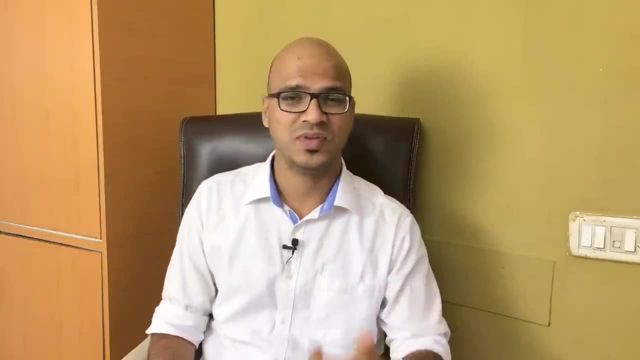 And, trust me, if you have ever worked on a software, you know how much documentation we have to create, And no one loves documentation, by the way. So we have a process, We have tools, We have documentation. This next thing is contract right. 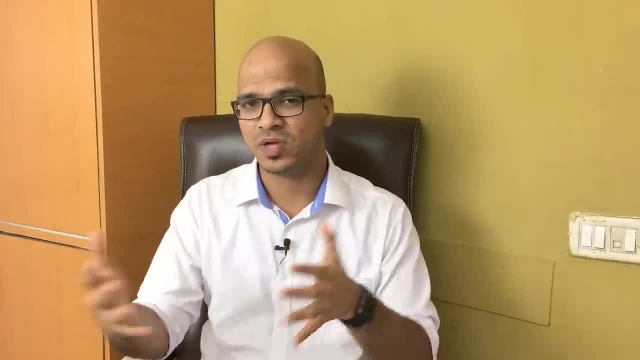 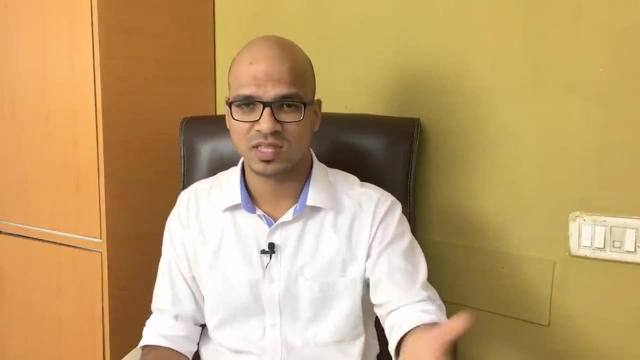 So, as a client, when you give a requirement for the vendor, they create a contract. This is what we will build Now, as a client, if you say we have to change something, they will show you the contract. This is the contract which you are working on, right? 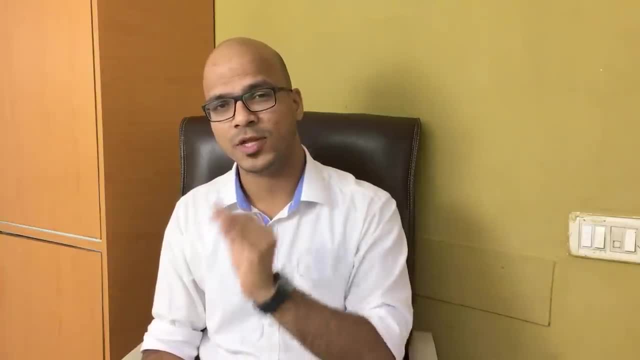 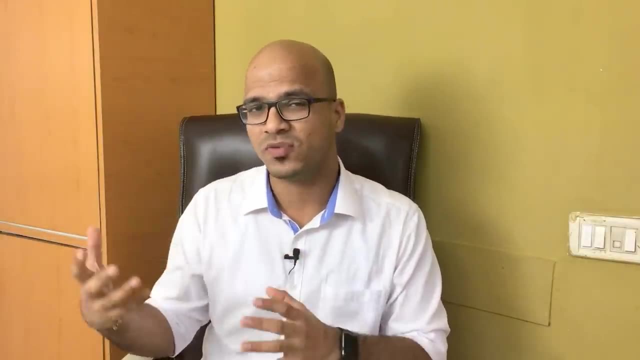 And in waterfall we always follow a particular plan. You cannot change the plan in between. So these are the some issues due to which there was some problem with the waterfall And to solve that, Agile is very simple. Agile says, okay, those things are actually important. 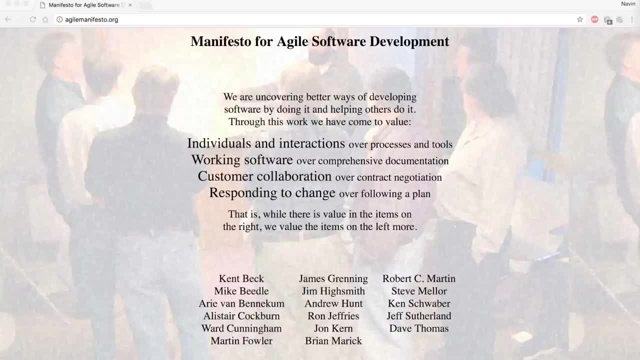 But more than that, we have four principles, or four values, So the values are. so, again, from where you will get these values? So, you will get these values from the actual website of Agile Manifesto. Okay, so the website name is agilemanifestoorg. 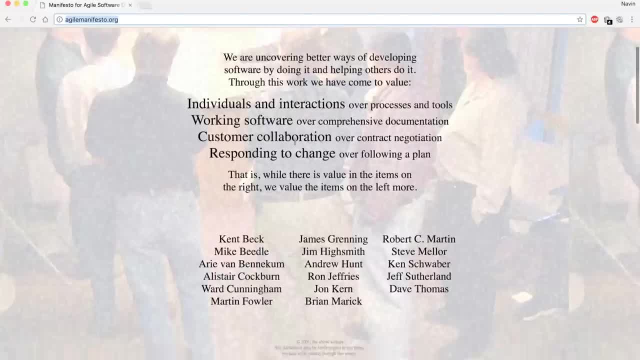 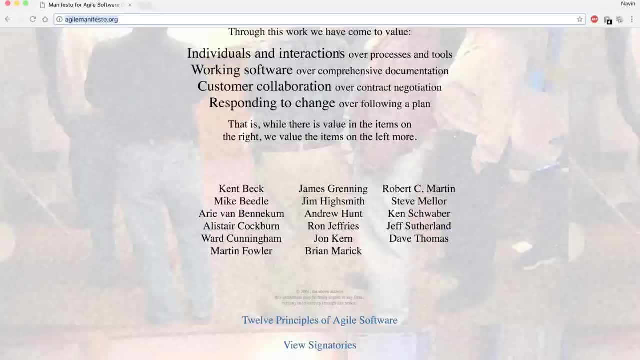 And it says it believes in. so there are two things: One is so you can see things on the right-hand side for you And the left-hand side. So things on the right-hand side are actually important, But not that important compared to left-hand side things. 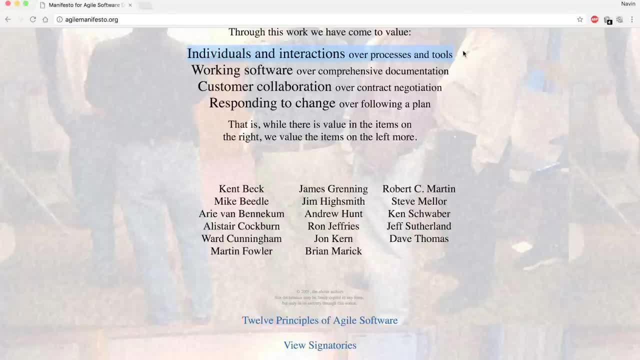 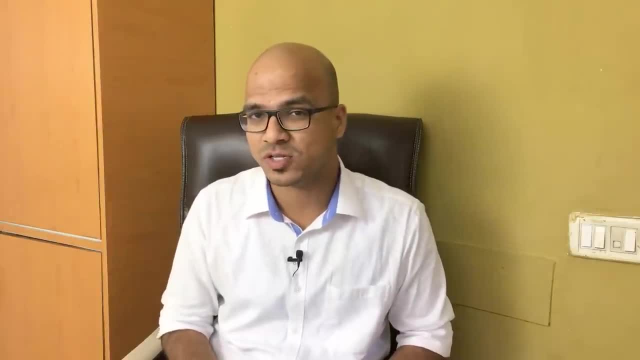 So it says individuals and interactions over process and tools. So you should give more importance to individuals and interactions, Because softwares are actually made by individuals, right? So you have to give them more importance And every person is different, right. 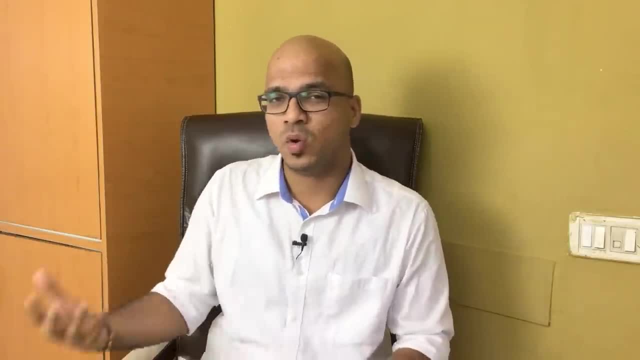 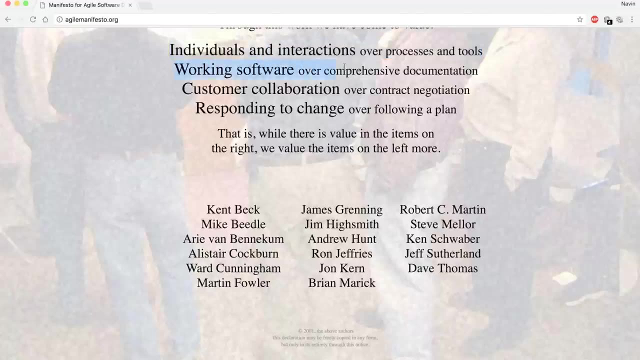 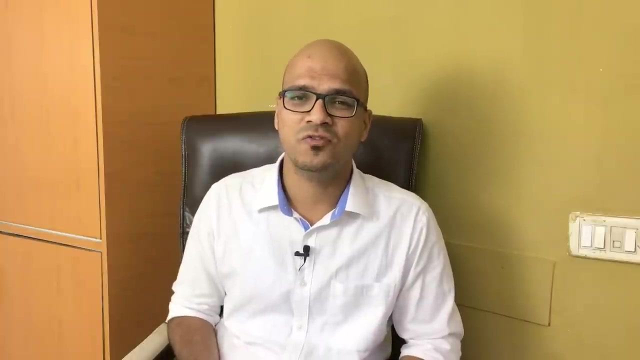 You cannot say two people will work in the same way, So they have their own what you say power. They have their own skill set. The next thing they talk about is focus on working software over comprehensive documentation And, of course, right when you buy a new phone, what you want. 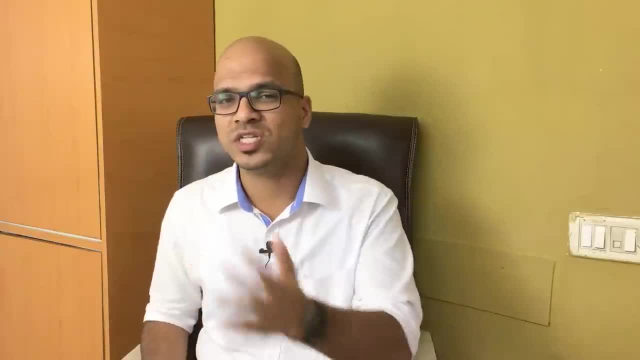 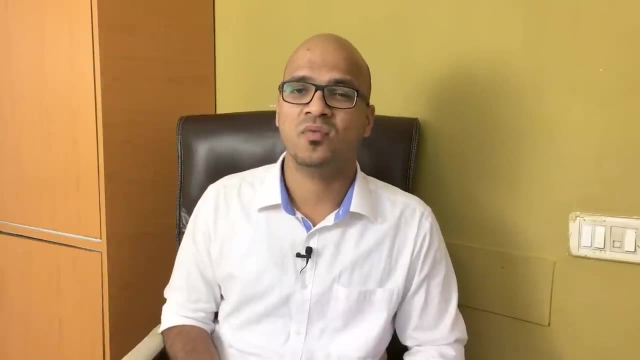 A working phone or a documentation which will teach you how to use phone. Of course, right, you want a working phone. So, in the same way, when you talk about softwares, you want a working software. You don't want a software which works, but not perfectly, but you have documentation to make it fix. 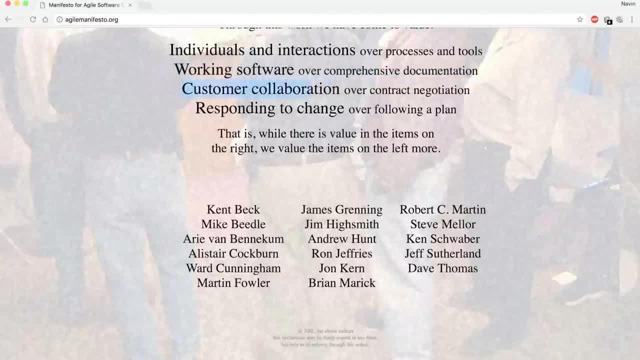 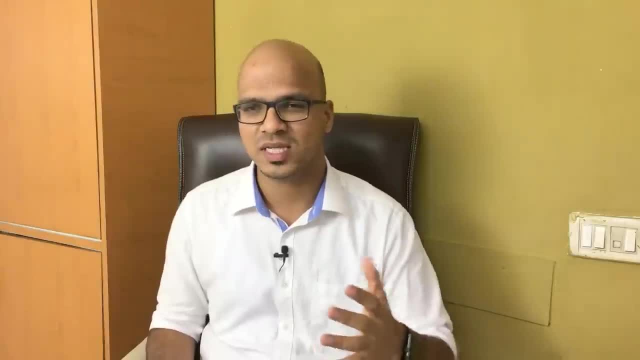 So the next, the third one, is customer experience, Customer collaboration over contract negotiation. So you have to focus more on customer collaboration. So if a customer says this is what we want, this is what we want, there should be a proper communication between you and a customer. 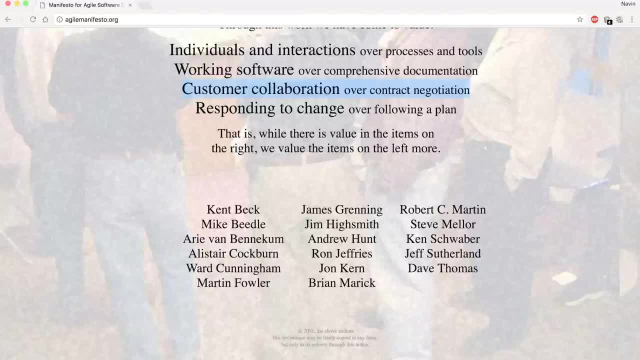 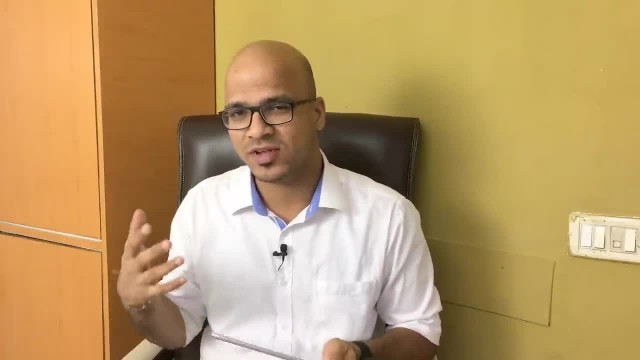 You should not focus on the contract, And the last one is respond to change over following a plan And, of course, right as a client. even a client don't know what he wants in the initial phase. So what you will do is: 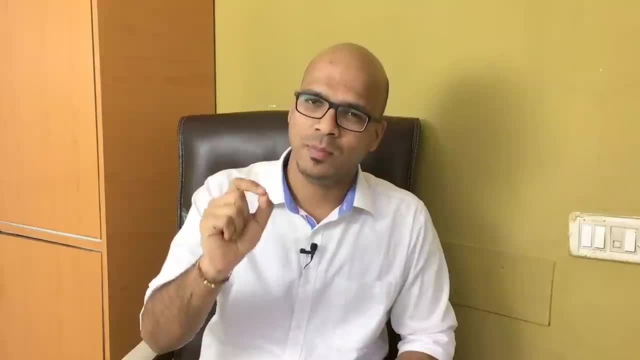 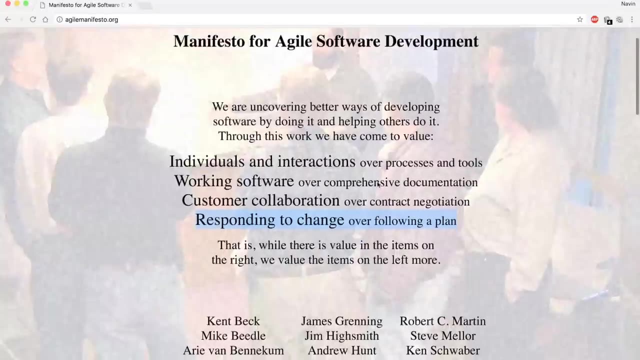 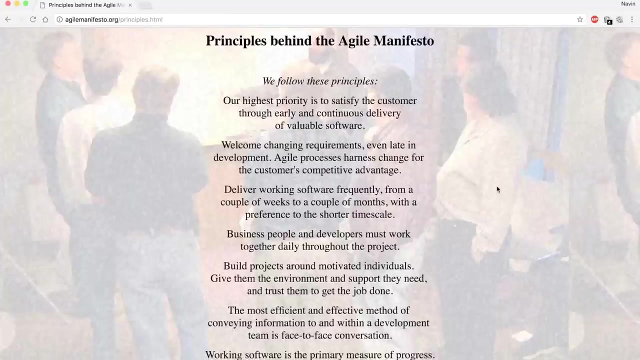 you will give a, you will give what you say MVP, which stands for Minimum Value Product, from which you will start building. So those are the four values. Now, with these four values, we also have 12 principles, And if you can implement these 12 principles in your project, you are being agile. 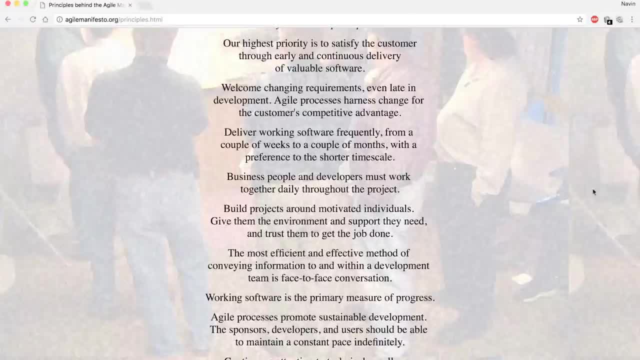 So what are those 12 principles? Again, it's a very lengthy one, so I will read it out as fast as possible. The first one is: our highest priority is to satisfy the customer through early and continuous delivery of value. So you have to provide this software in a continuous manner. 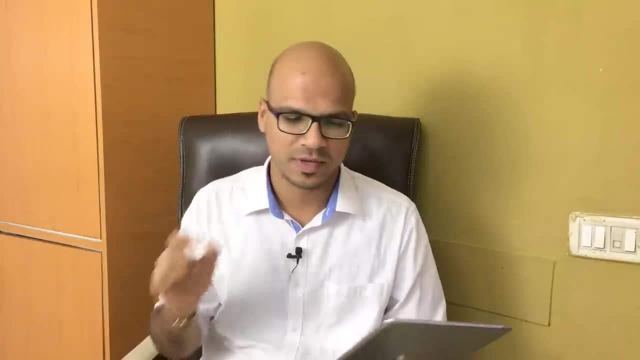 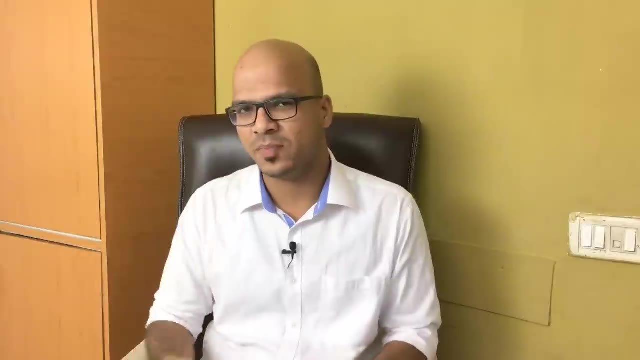 not as a one-go, not as a big bank software, but in continuous delivery. Next, welcome changes requirement even late in development. So let's say, after building half of the project, if a client says, okay, we want this new feature, you should not say no. 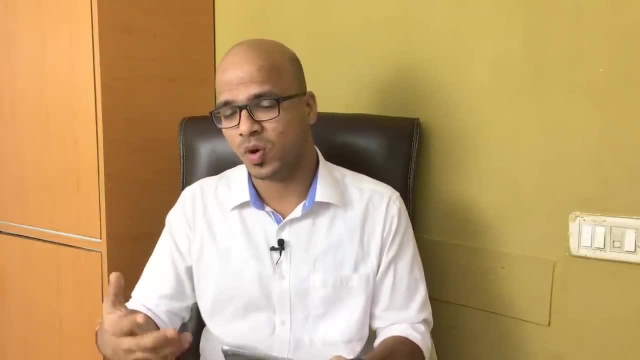 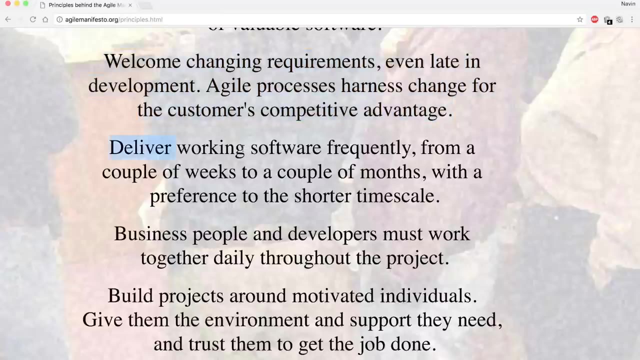 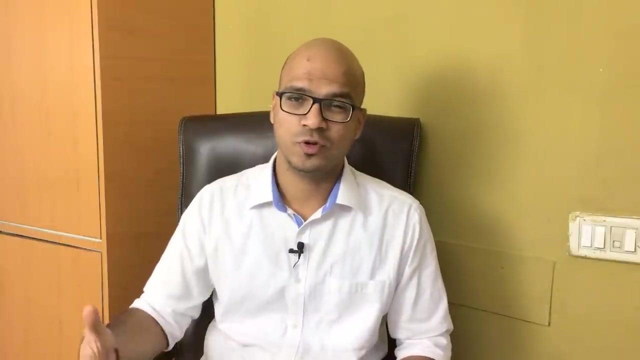 You are a person and you are a development team who is providing service to the client, So you have to provide, you have to accept the changes. Next, delivery working software frequently from a couple of weeks to a couple of months, So don't ask your client to wait for two years or three years. 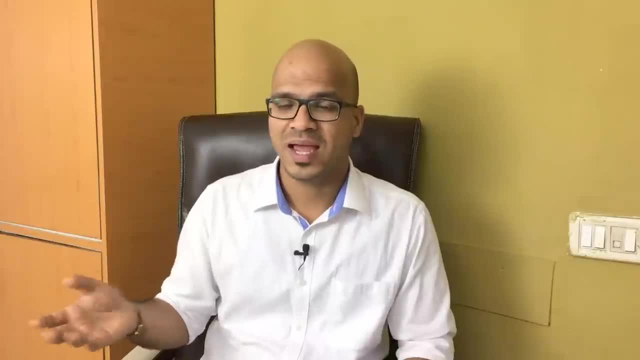 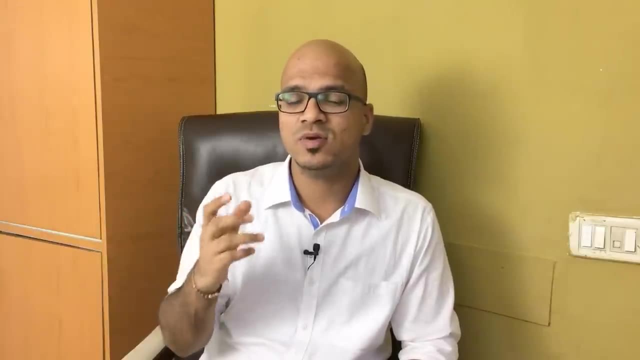 You have to deliver the software in every two to four weeks And if you are implementing this using Scrum, so Scrum is actually a framework using which you can implement agile. So in Scrum we use a term called as Sprint. So Sprint is basically two to four weeks time span where you have to deliver the product. 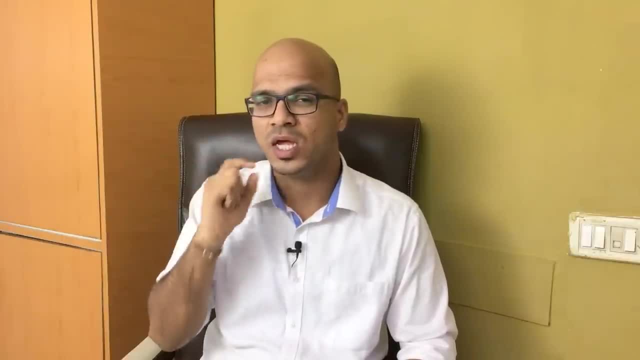 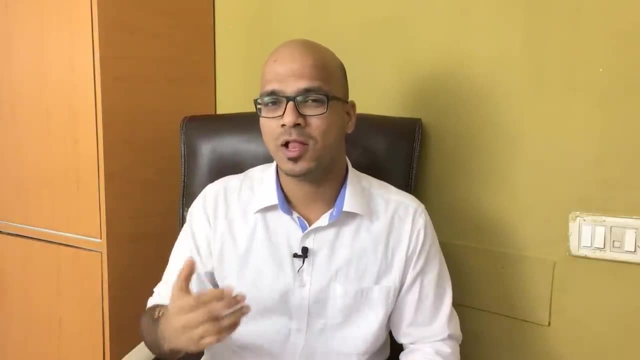 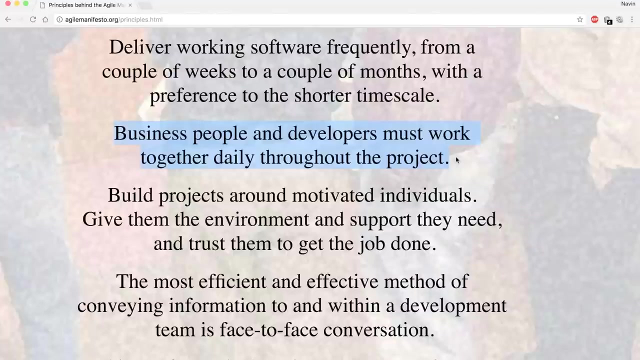 So after every Sprint, or after every two to four weeks, you should be giving a software to the client which will be called as potentially shippable product. Okay, next one is business. people and developers must work together daily throughout the project. 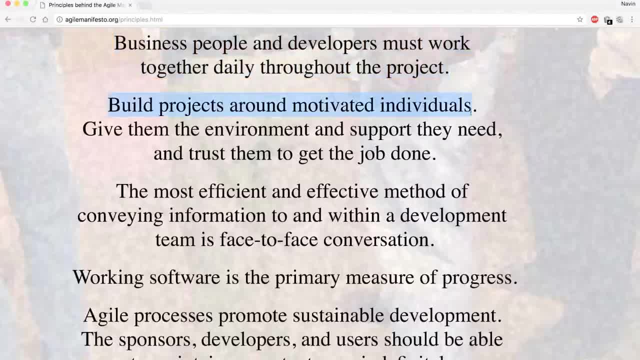 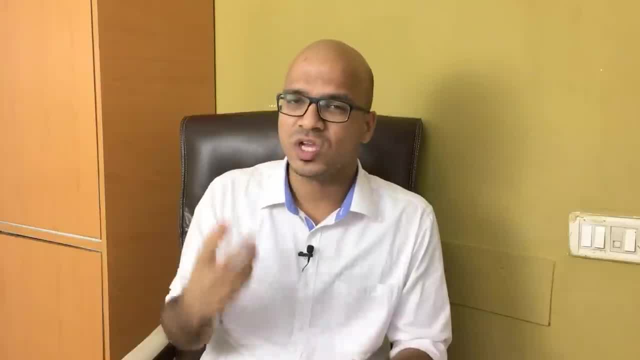 And that makes sense right. Next one is build projects around motivated individuals. give them the environment and support they need and trust them to get the job done. You have to give importance to individuals, right? Don't focus more on process. You have to focus more on individuals. 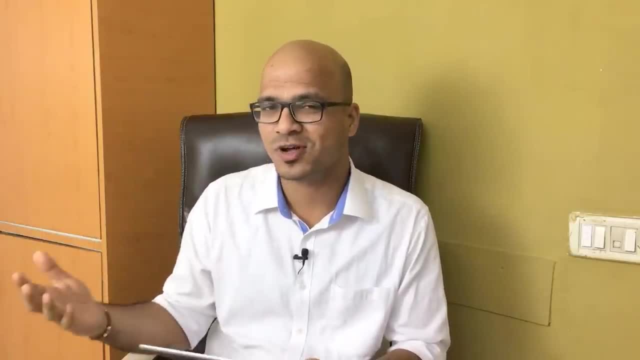 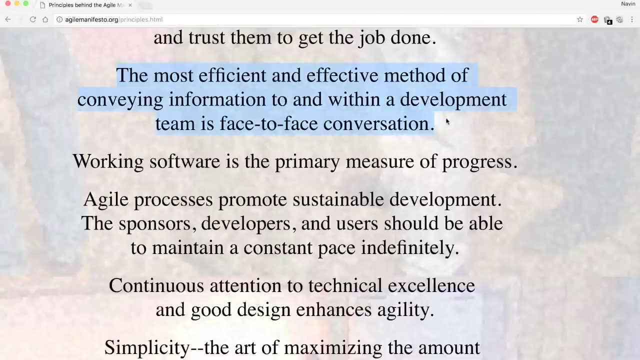 That doesn't mean that you should not focus on process as well. You should focus that, but then give more importance to individuals. So next one is: the most efficient and effective method of conveying information to and within the development team is to face-to-face conversation. 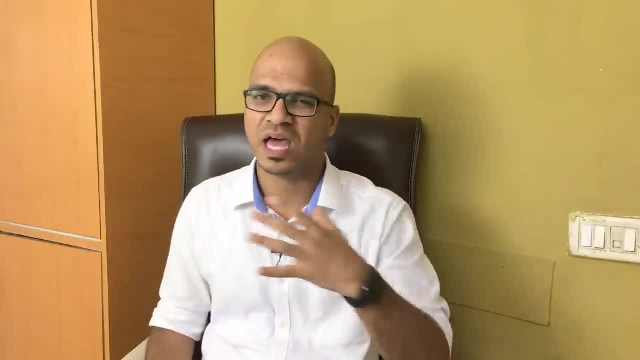 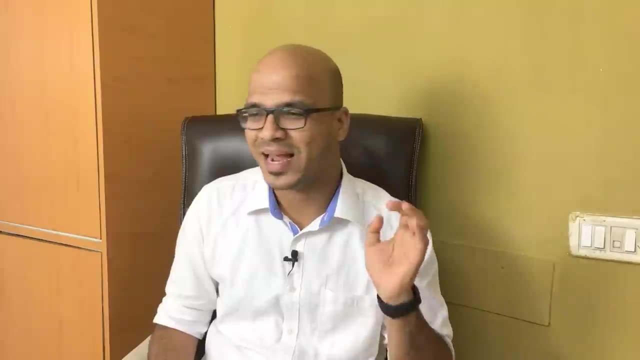 You know, earlier days people used to discuss because we have on-site team, we have off-site team and so we'll be having a big team. The problem is they normally talk on phone And that's the weird way of communication, because if you're interacting with someone on phone, 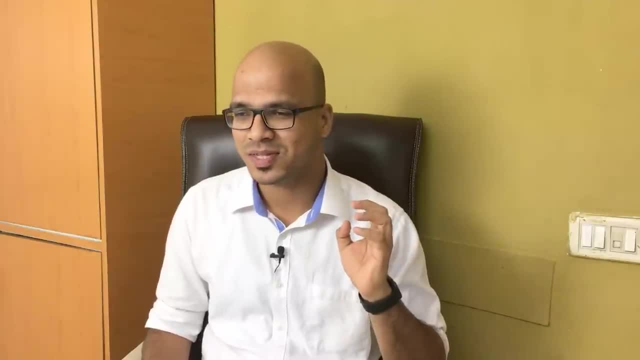 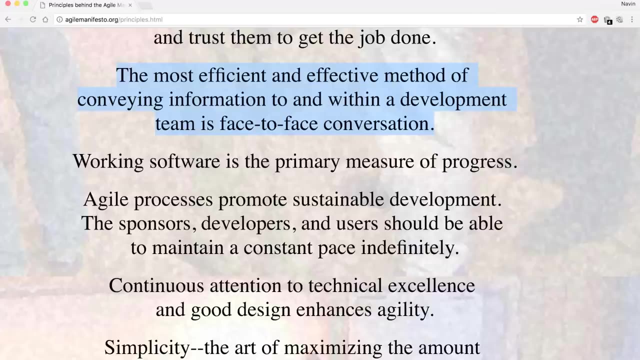 that's where the problem starts, right, Because it's very difficult to convey something over a phone, right? So having a face-to-face conversation or maybe a video call will be much better. The next one is working. software is a primary measure of progress. 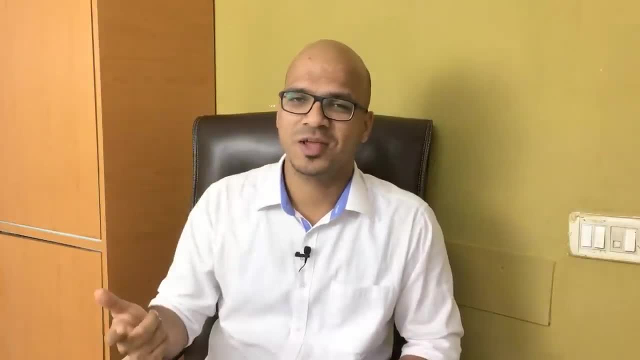 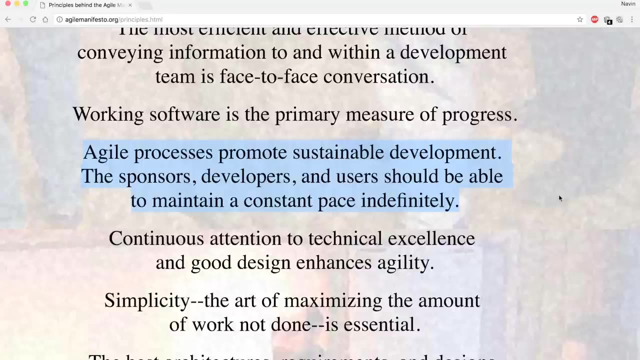 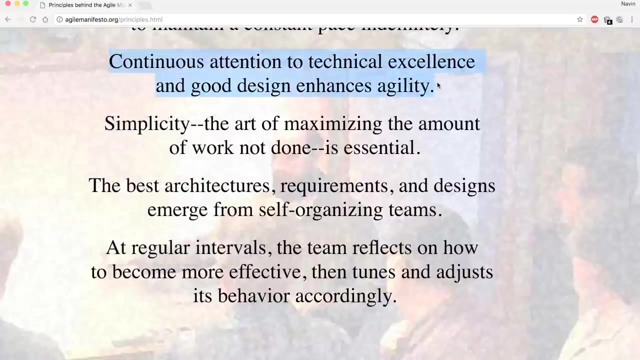 How do you check your progress? Best thing is check the working module right. Next one is agile processes: promote sustainability. agile development, the sponsors, developers and users should be able to maintain a constant pace indefinitely. Next is continuous attention to technical excellence and good design: enhance agility. 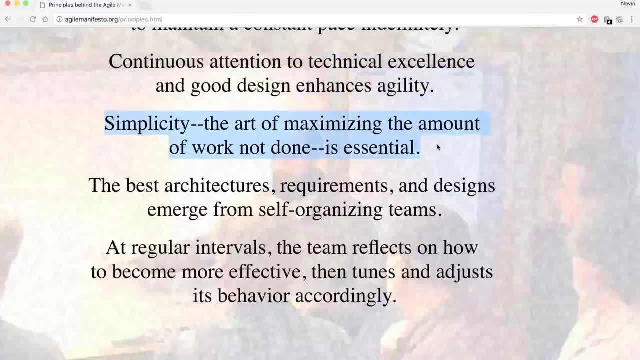 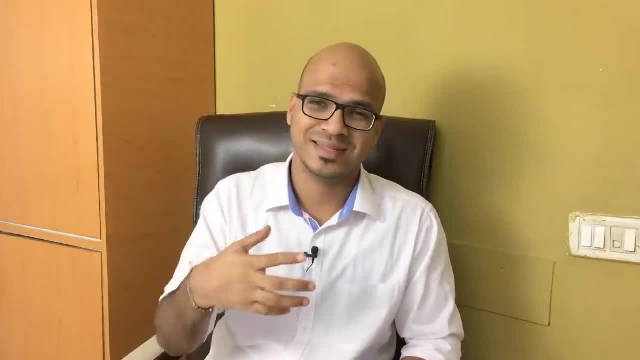 The next one is simplicity, The art of maximum the amount of work not done is essential Because when you work on a project, there are some modules which are very important, there are some modules which are not that important. You have to skip those things which are not important. 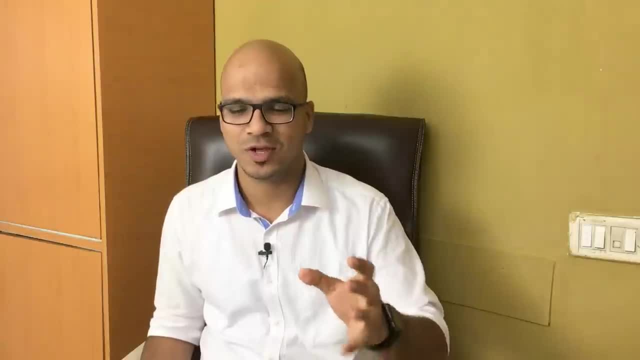 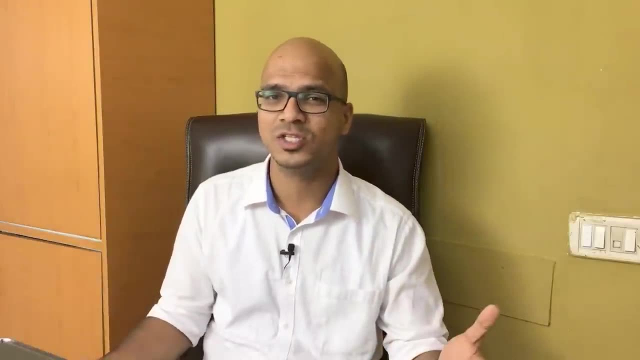 But normally what we do is, you know, when you work on a project you think, okay, this is the feature which we can add, this is something which we can add, and those things get increment and you get a very bulky software and you get most of the features which you don't even want. 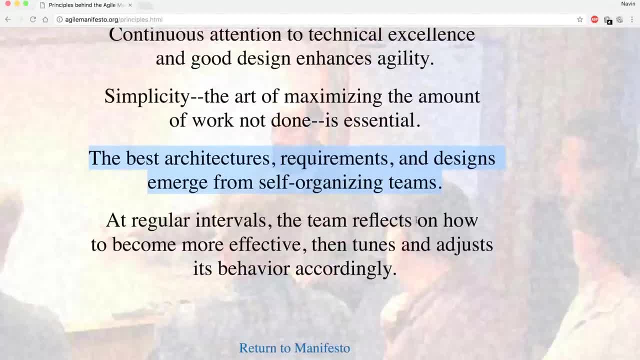 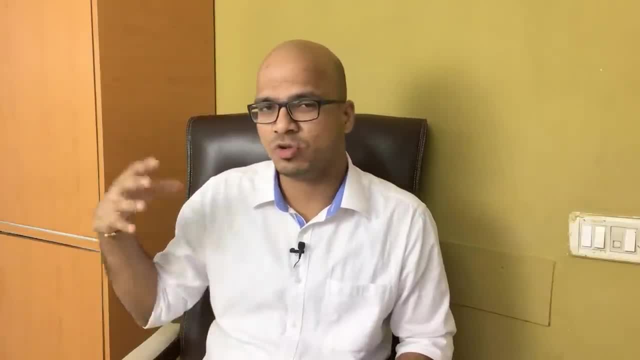 The next one is the best architectures, requirements and design emerge from self-organizing team. So in agile, you want your team to be self-organizing, which simply means that there should not be someone who will force them to do it. 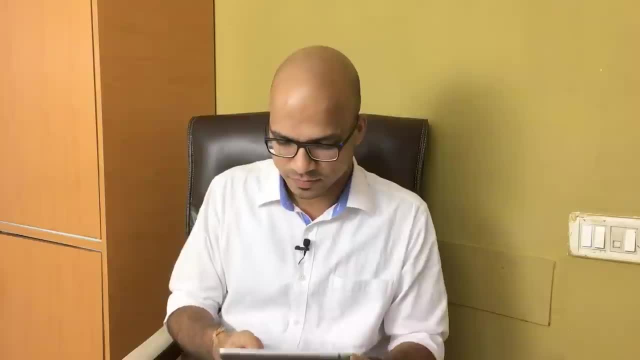 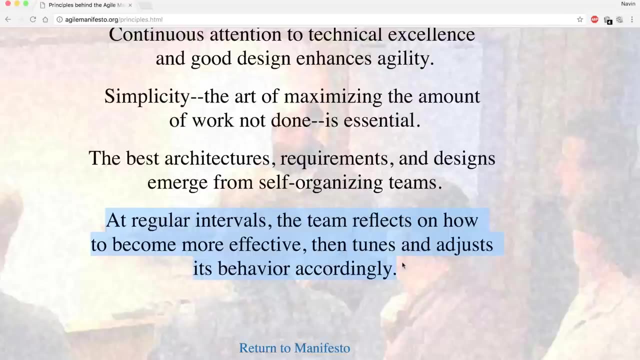 Your team should know what to do and how to deliver the product, Because it's not easy, Because it's not an individual effort, it's actually a team effort. Next one is: at a regular interval, the team reflect on how to become more effective. 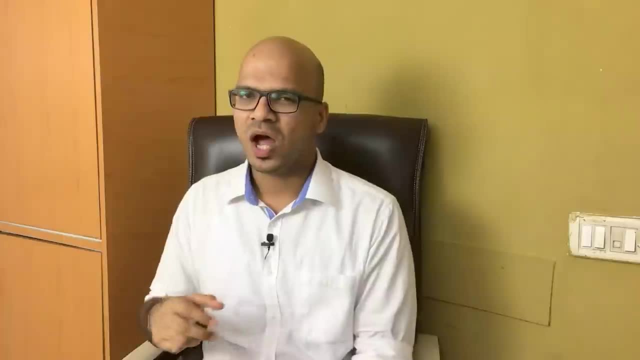 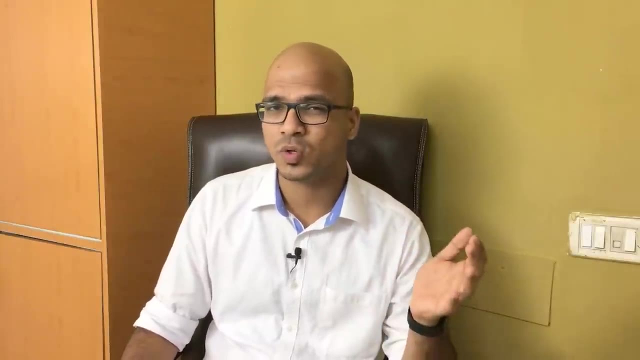 then tunes and adjust in behavior accordingly. So after every sprint you know if you talk about scrum. after every sprint you have to make sure that they are. they should check what's going right and what's going wrong so that they can improve their performance for the next sprint. 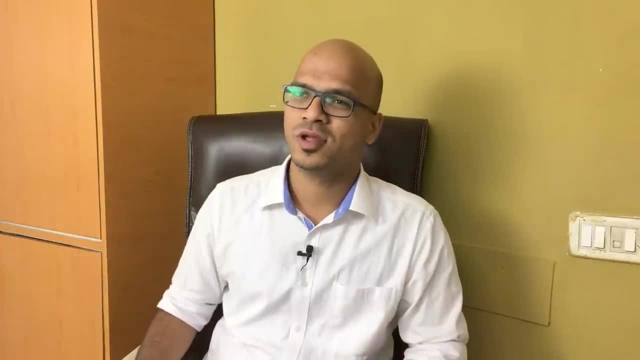 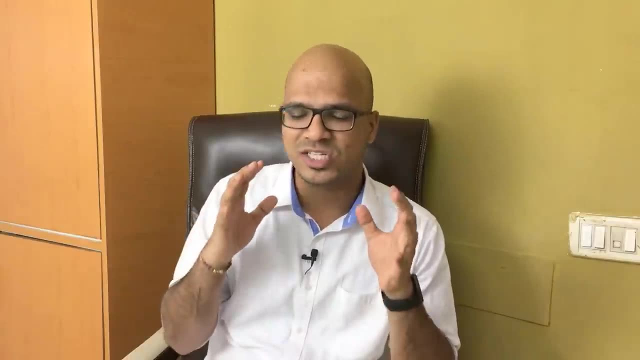 So if you follow these 12 principles and if you follow those 4 values, you are being agile. Now, it's not actually a methodology. okay, Agile is not a methodology, it's a philosophy. So if you follow these things, you are good to go.